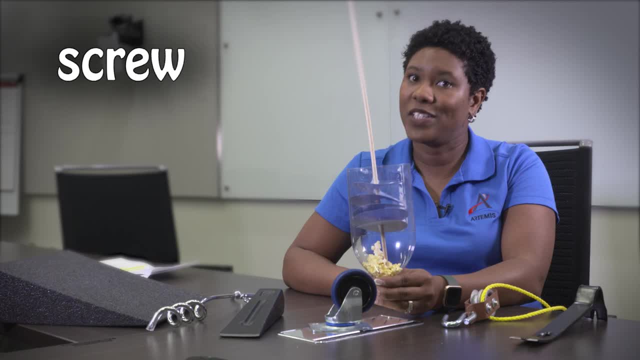 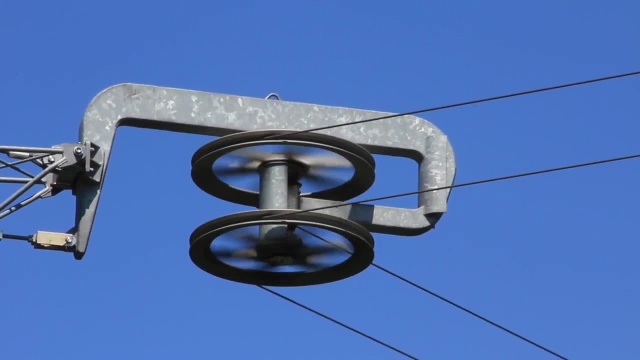 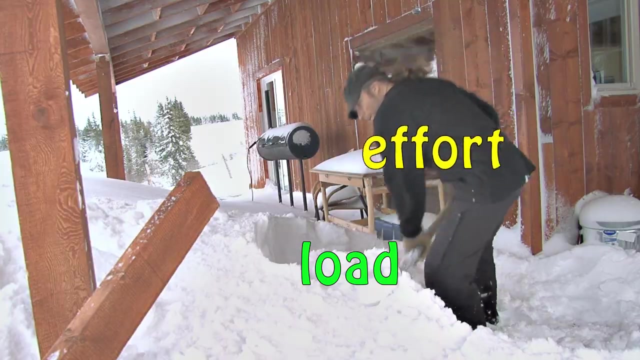 a pulley and a lever. If you guessed the screw, you're correct. A simple machine is a tool that can help you do work easily. Simple machines have one to two parts. They can make a force stronger, change the direction of a force or change the speed of a force. The force you apply is called the effort. 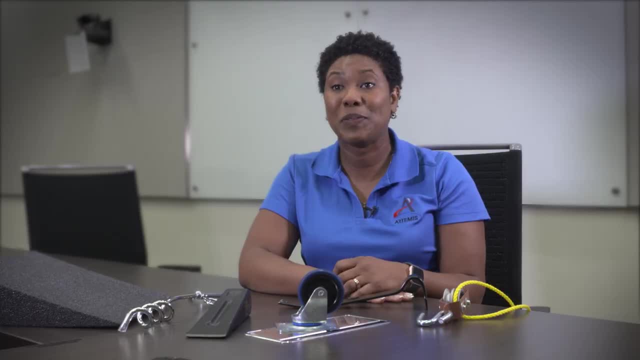 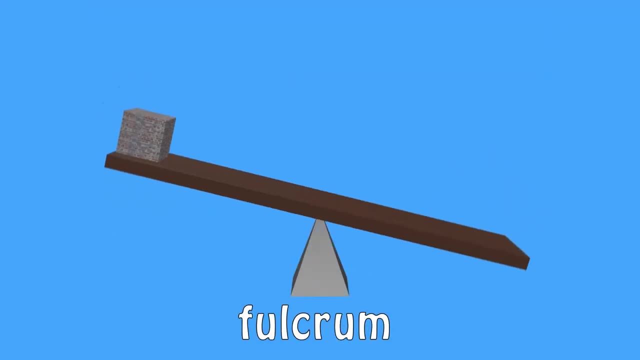 The object you move is called the load. There are two groups of simple machines. One group is a lever. A lever is a straight bar that moves on a pivot point called a fulcrum. It helps you to lift something. The object lifted is called the load. The closer the object, 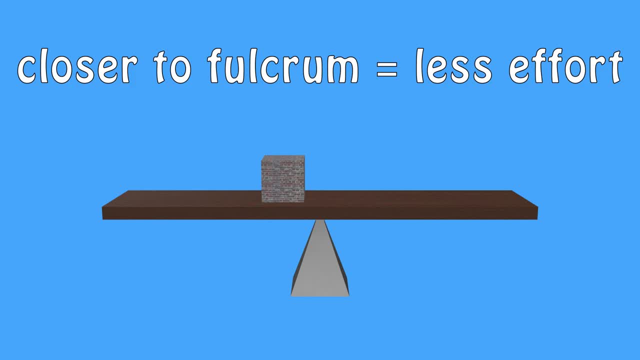 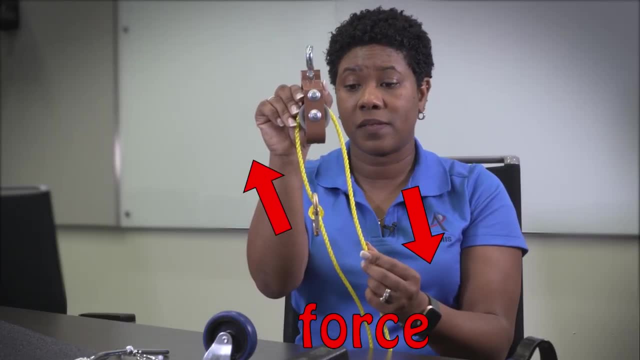 is to the fulcrum, the less effort that's needed to lift the object. A pulley is another type of lever. It's made of a rope and a wheel. When you pull down on the rope, it changes the direction of the force causing the object on the other side. 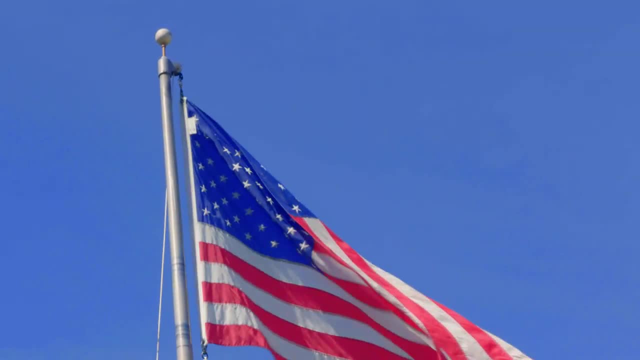 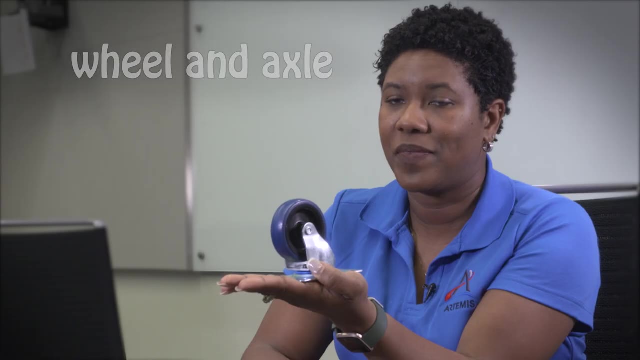 to rise. An example is a flagpole. You may have seen one outside of a school. Another type of lever is called a wheel and axle. It's made of a wheel attached to a post called an axle. It also helps to make work easier. I'm sure you can think of lots of examples. 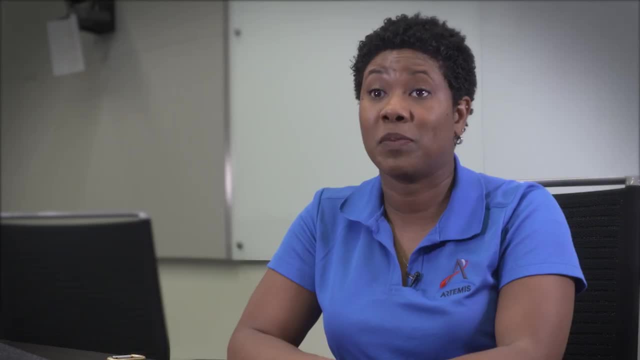 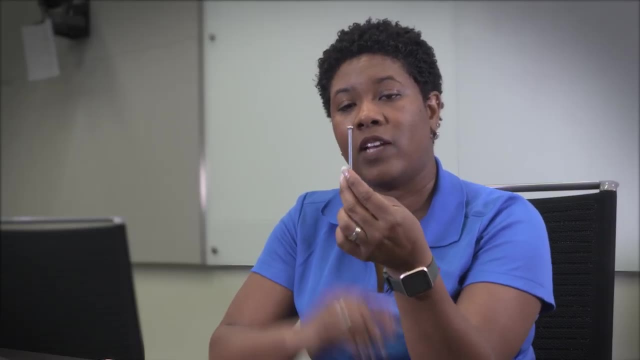 of wheel and axles all around you. The second group of simple machines are called incline planes. They make work easier by reducing the amount of effort needed to move an object. A screw is an inclined plane wrapped around a cylinder, It turns a turning force into a vertical force. 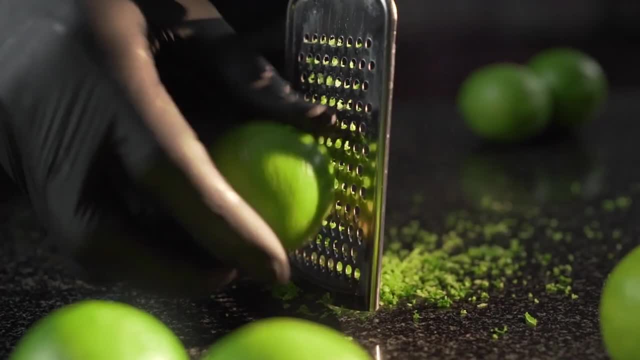 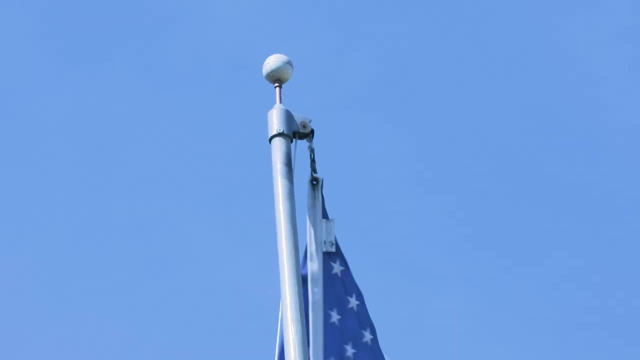 A wedge is made of two inclined planes back to back and we use it to split objects apart. Sample machines are all over our daily lives, like a seesaw flagpole, window blinds, toy cars, office chairs, slide wheelchair ramp. 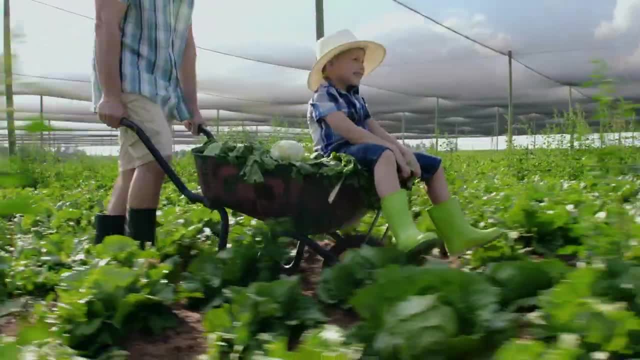 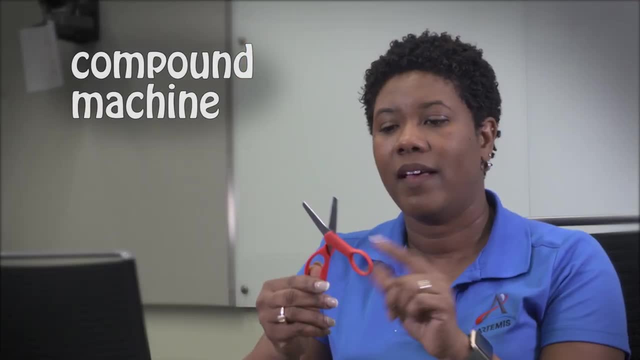 jar lid, a light bulb, a knife or a shovel or a wheelbarrow. Sometimes two simple machines can be combined to create a compound machine like scissors. They are two wedges and two levers. Together they help cut paper. 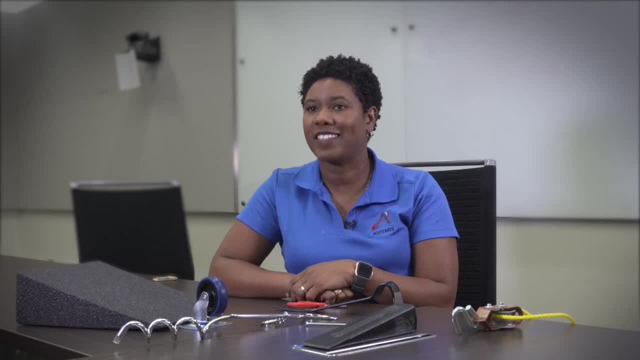 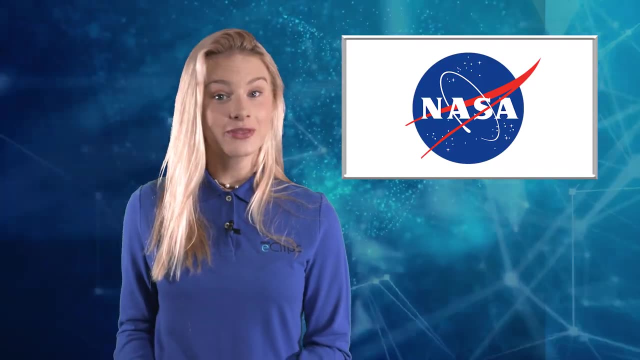 As you can see, simple machines really are all around us. Wedge-o, look at that. Simple machines are really all around us. But did you know that NASA uses simple machines too? NASA uses simple machines for many applications, For example, like Lunar Crane.